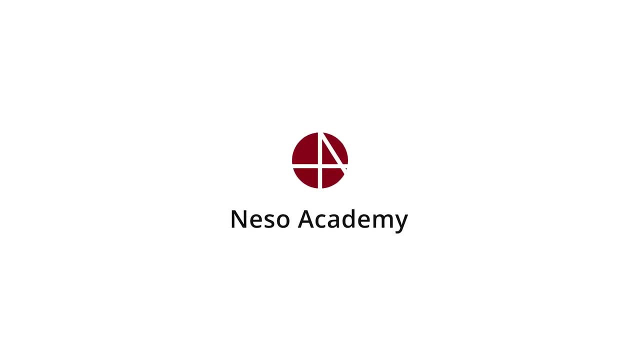 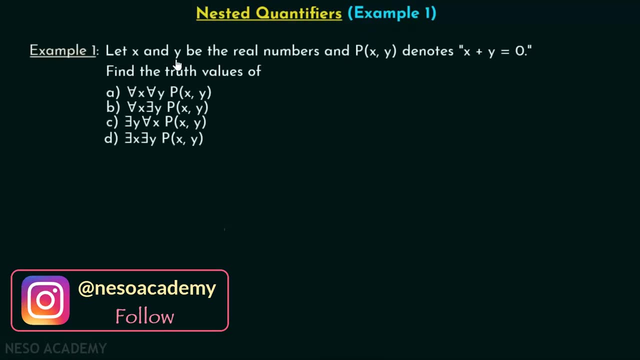 Let's consider example 1 on nested quantifiers. Let x and y be the real numbers, and p x comma y denotes x plus y is equal to 0.. Okay, so this is the propositional function: p x comma y, which denotes x plus y is equal to 0. 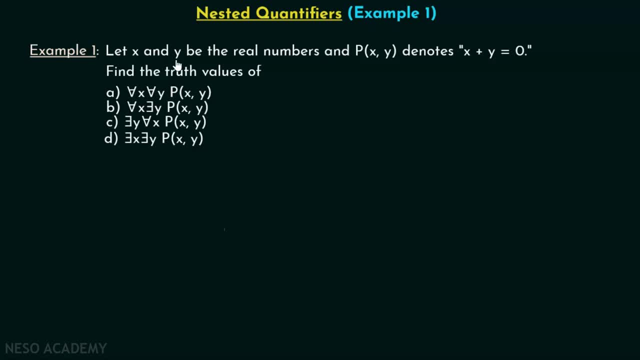 and domain consists of all real numbers. We are considering two variables, x and y. here, as you can see right, Find the truth values of: for all x. for all y, p x comma y. for all x. there exists y, p x comma y. there exists y. for all x. p x comma y. there exists x. there exists y, p x comma y. 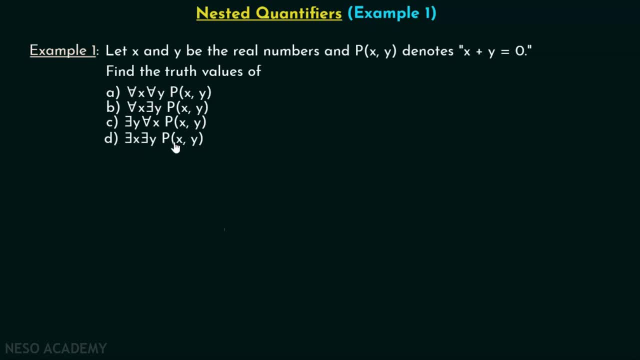 These are all the options. We need to find the truth value of all of them. Okay, now we know that domain consists of all real numbers. right, Let's consider part a, that is, for all x, for all y, p, x, comma, y. 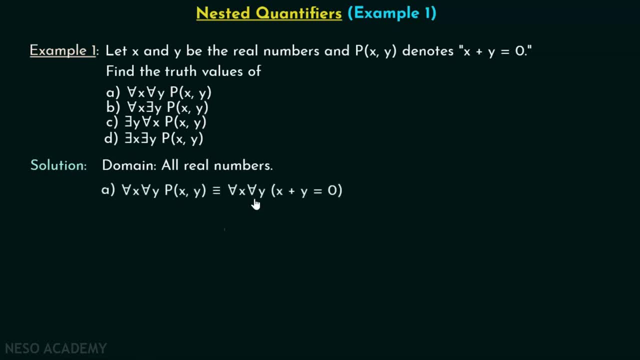 We can write this: for all x for all y: p x comma y. as for all x for all y: p x comma y. as for all x for all y: x plus y equal to 0.. Instead of writing p x comma y, I can write x plus y equal to 0.. 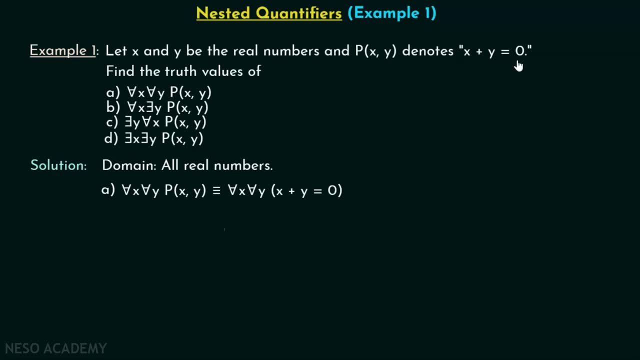 We know that p x comma y denotes x plus y is equal to 0, right? That is why I can replace this p x comma y by x plus y, equal to 0.. Now, what does this mean For all real numbers, x and y? x plus y is equal to 0. 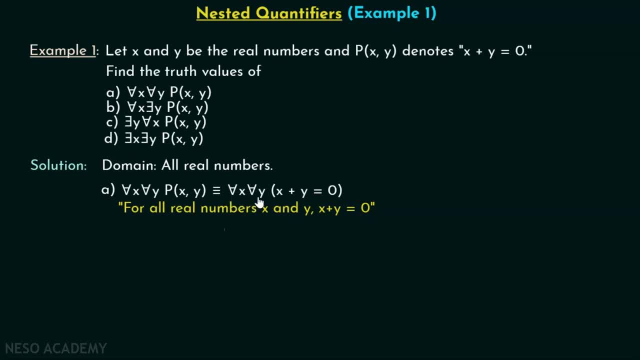 For all real numbers x and for all real numbers y. x plus y is equal to 0.. Please note that domain consists of all real numbers. It is given in the question. We know that x and y are real numbers. Here we can say that for all real numbers x and for all real numbers y. 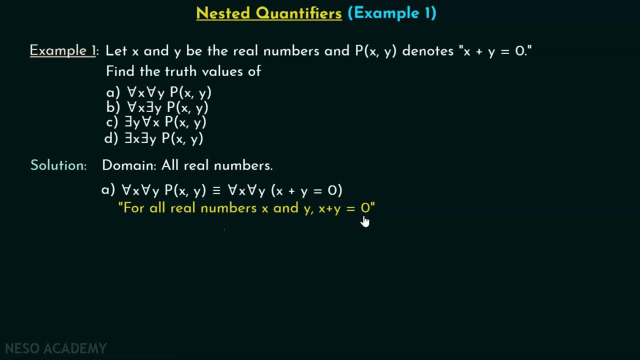 or for all real numbers, x and y, x plus y is equal to 0.. Now, is it true? Can you say this is true? No, this is not true. Think of it as for any combination of x and y, p, x, comma, y. 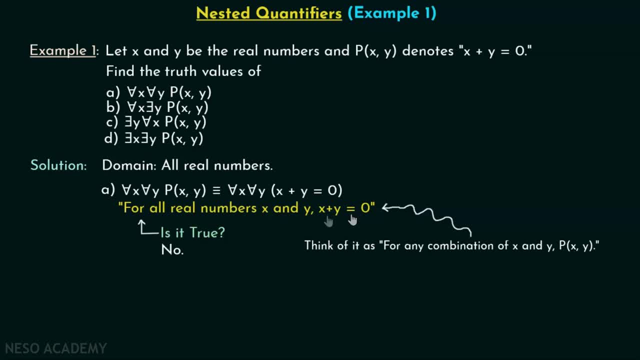 Let me tell you that for 1 and minus 1, this is true. 1 plus minus 1 is actually equal to 0. But what about 1 plus 2? 1 plus 2 is not equal to 0, right. 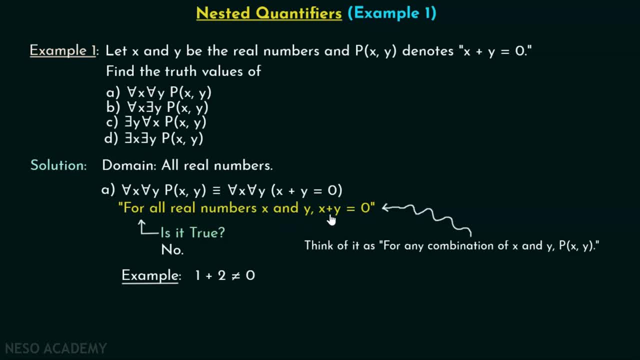 So it is clear from this fact that for all real numbers, x and y, x plus y is not equal to 0.. Also, for all y, for all x, p, x, comma y is actually equivalent to for all y, for all x, x plus y equal to 0.. 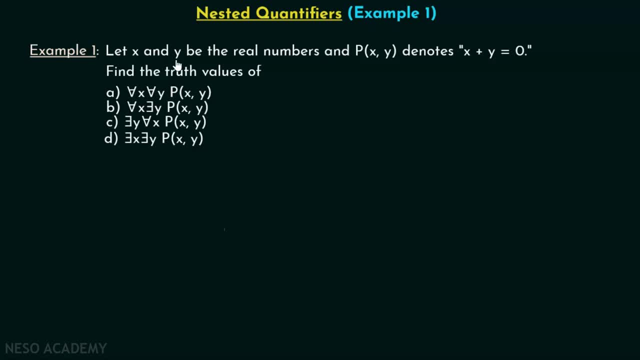 and domain consists of all real numbers. We are considering two variables, x and y. here, as you can see right, Find the truth values of: for all x. for all y, p x comma y. for all x. there exists y, p x comma y. there exists y. for all x. p x comma y. there exists x. there exists y, p x comma y. 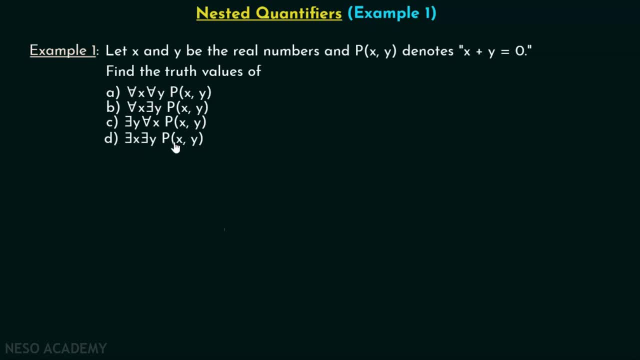 These are all the options. We need to find the truth value of all of them. Okay, now we know that domain consists of all real numbers. right, Let's consider part a, that is, for all x, for all y, p, x, comma, y. 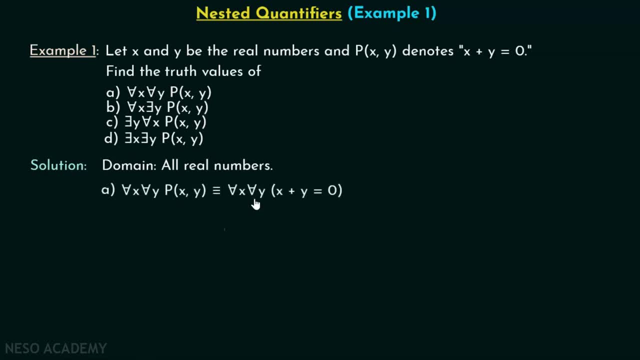 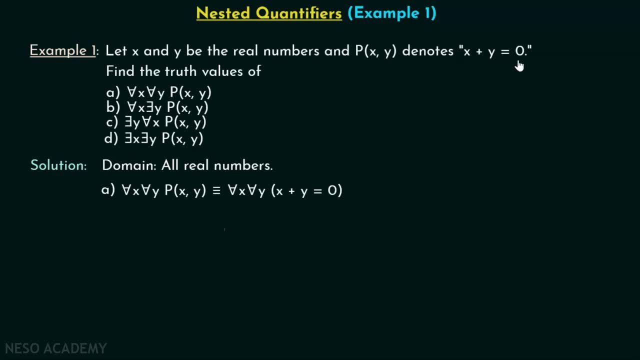 We know that p x comma y denotes x plus y is equal to 0, right? That is why I can replace this p x comma y by x plus y, equal to 0.. Now, what does this mean For all real numbers, x and y? x plus y is equal to 0. 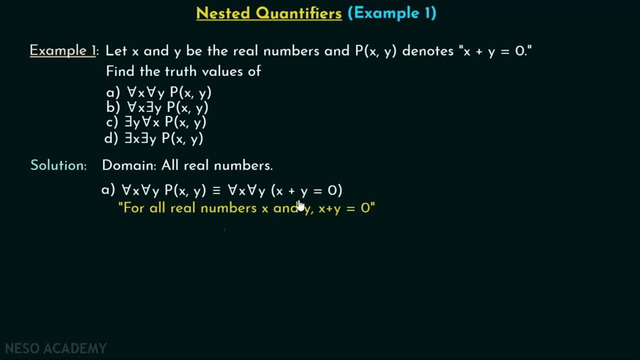 For all real numbers x and for all real numbers y. x plus y is equal to 0.. Please note that domain consists of all real numbers. It is given in the question itself. We know that x and y are real numbers. Here we can say that for all real numbers x and 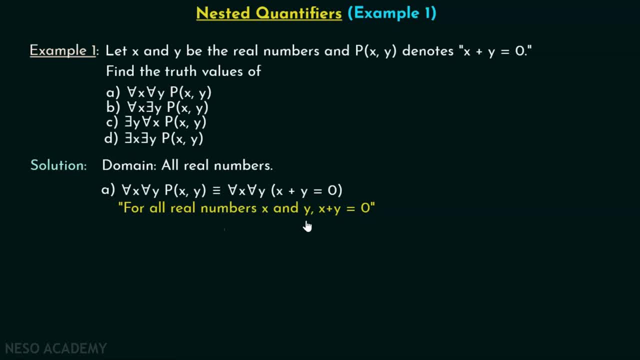 for all real numbers y, or for all real numbers x and y. x plus y is equal to 0. Now, is it true? Can you say this is true? No, this is not true. Think of it as for any combination of x and y. 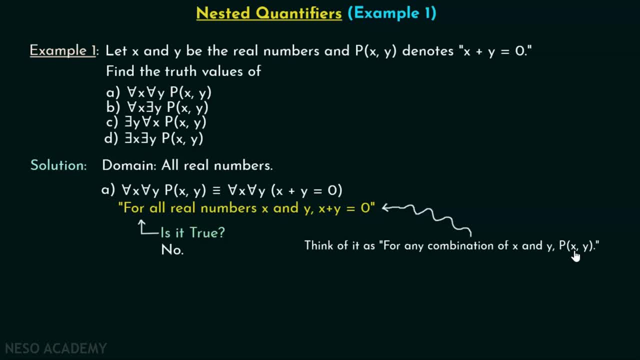 px, comma y, Let me tell you that for 1 and minus 1, this is true. 1 plus minus 1 is actually equal to 0.. But what about 1 plus 2? 1 plus 2 is not equal to 0, right? So it is clear from this fact. 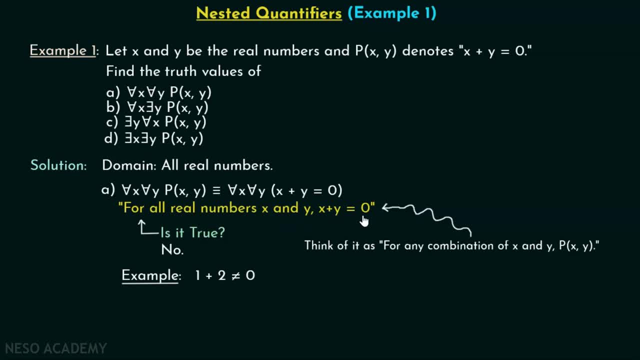 that for all real numbers, x and y, x plus y is not equal to 0.. Also, for all y, for all x, px, comma y is actually equivalent to: for all y, for all x, x plus y equal to 0, which can be written as for: 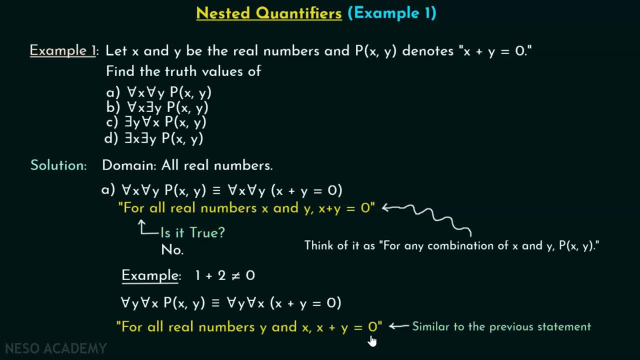 all real numbers, y and x, x plus y is equal to 0, which is similar to this statement: right For all real numbers, x and y, x plus y is equal to 0.. So it is clear from this fact as well. 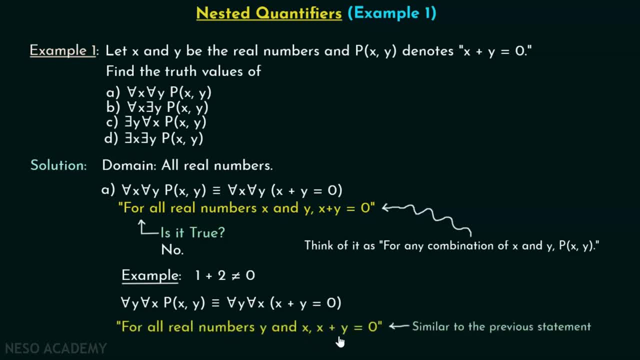 Which can be written: as for all real numbers, y and x, x plus y is equal to 0.. Which is similar to this statement: right, For all real numbers, x and y, x plus y is equal to 0.. So it is clear from this fact as well that for all y, for all x. 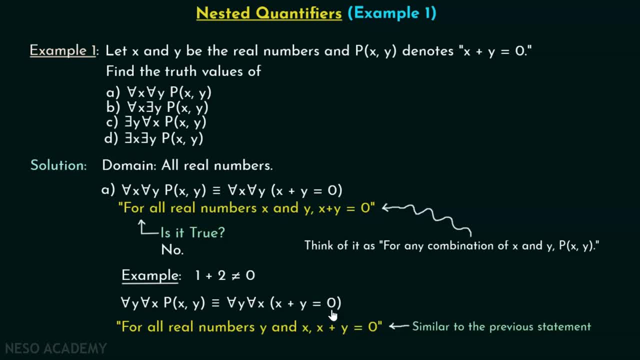 x plus y is not equal to 0.. Okay, So the truth value for the first part, that is for all x, for all y, p, x, comma y, is actually false. Okay, Now let's consider part b, that is for all x. there exists y, p, x comma y. 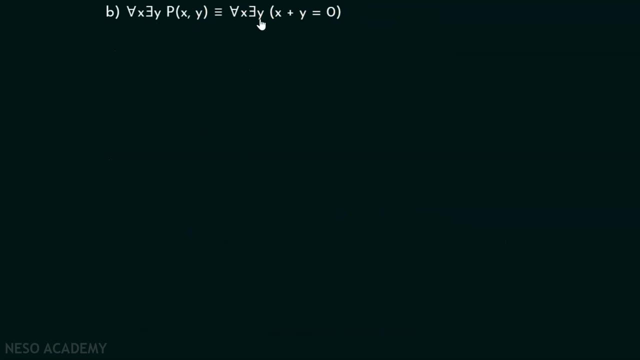 For all x, there exists y, p, x comma y can be written: as for all x, there exists y. x plus y equal to 0.. Now how to read this statement? For every real number x, there exists a real number y, such that x plus y equal to 0.. 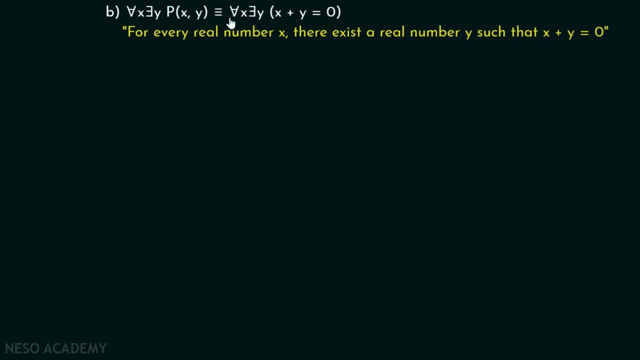 Isn't that? so We know that y depends on x. right, For every real number x, there exists a real number y, such that x plus y is equal to 0.. Now let me tell you that this is true, right. 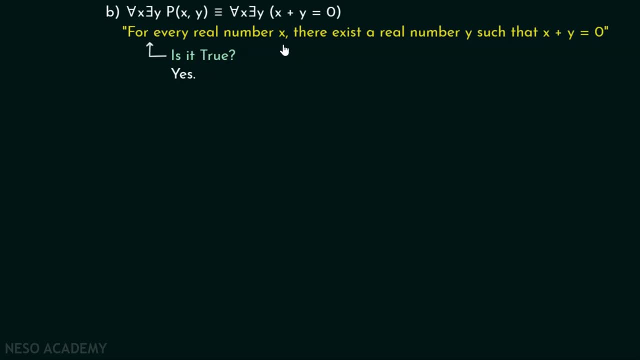 We can say that this is true Because for every real number x, there is at least one real number y, for which x plus y is equal to 0.. Right, You can choose any real number x, there is always a real number y for that x, right? 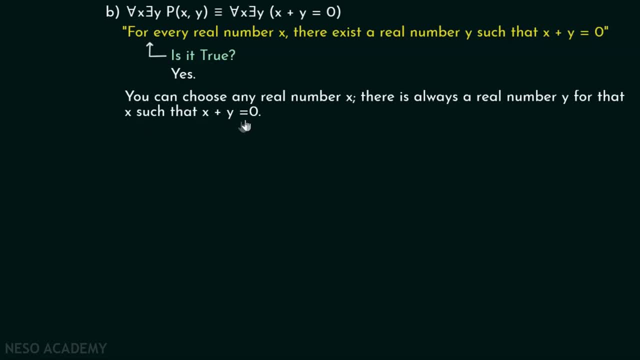 Such that x plus y is equal to 0.. Please note that We can choose any real number x. it is our choice. There is always a real number y for that x, such that x plus y is equal to 0.. For example, you can consider x equal to 1.. 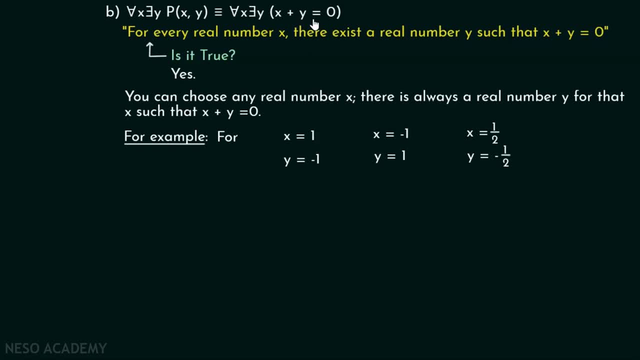 You know that for x equal to 1, there is a y which makes x plus y, 0,. right, We can choose y as minus 1.. Let's say, if we select x equal to minus 1, then we have y equal to 1.. 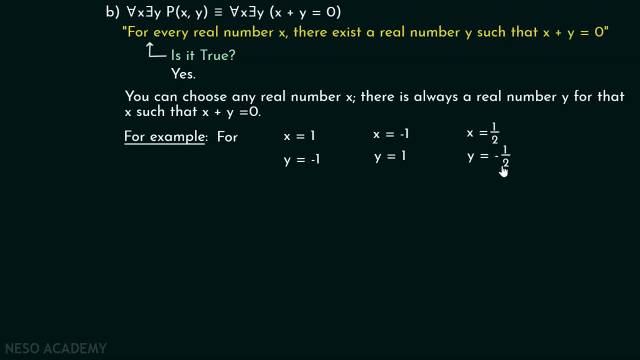 If we choose x equal to 1 by 2, then we have y equal to minus 1 by 2.. Now you get it: Y. for every real number x there exists a real number y, such that x plus y equal to 0 is true. 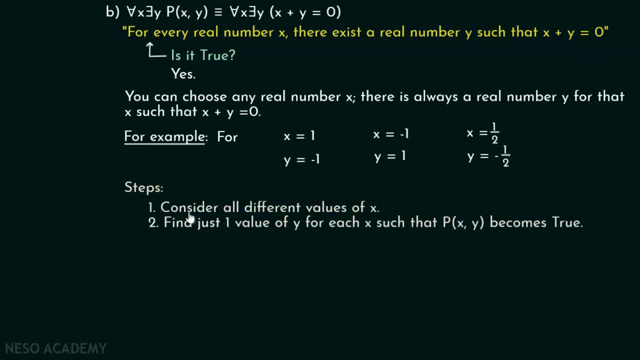 Right, If you are confused, then you can follow these steps. Consider all different values of x. Okay, You should consider all different values of x, because it is for all x Right Now. you just have to find one value of y. 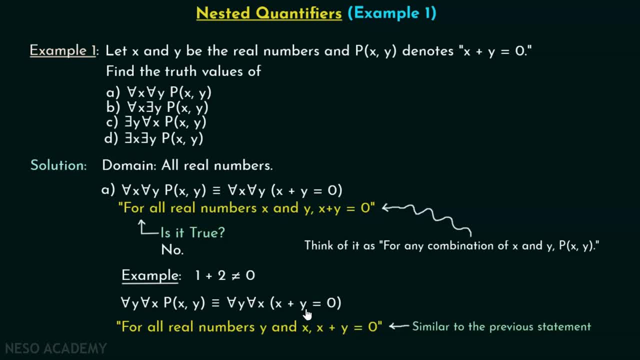 that for all y, for all x, x plus y is not equal to 0,. okay, So the truth value for the first part, that is, for all x, for all y, px, comma y is actually false. okay, Now let's consider part. 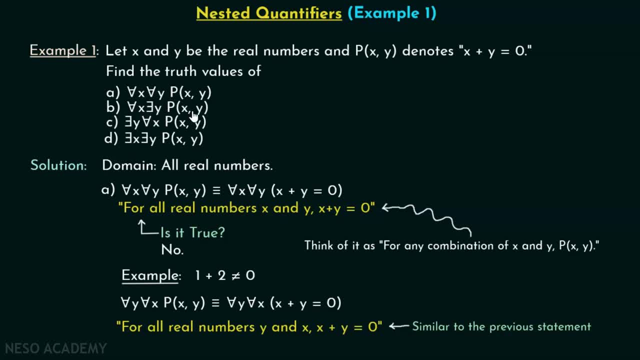 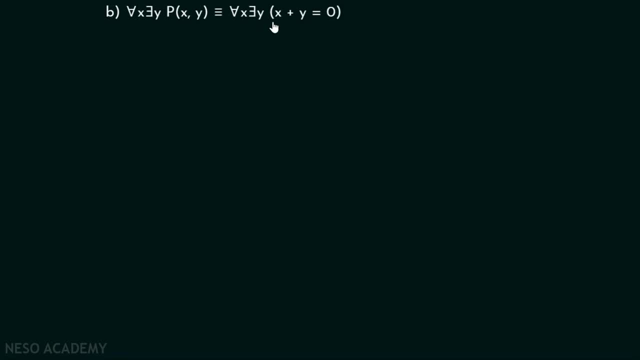 b. that is, for all x there exist y px comma y. For all x there exist y px comma. y can be written: as for all x, there exist y, x plus y equal to 0.. Now how to read this statement For every real 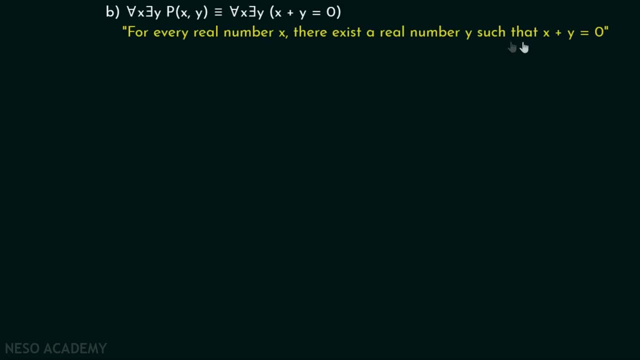 number x, there exist a real number y. For every real number y, there exist a real number y, Such that x plus y equal to 0.. Isn't that so We know that y depends on x, right For every real. 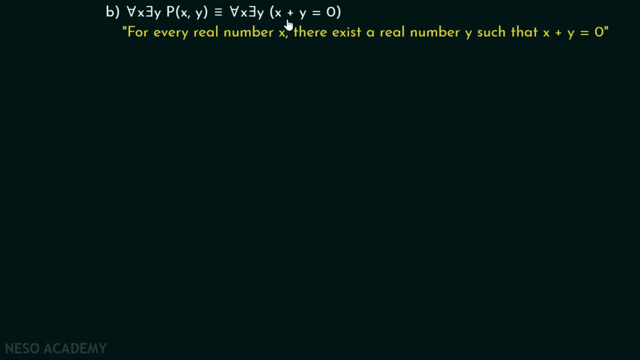 number x, there exist a real number y, such that x plus y is equal to 0.. Now let me tell you that this is true. right, We can say that this is true because for every real number x, there is at least 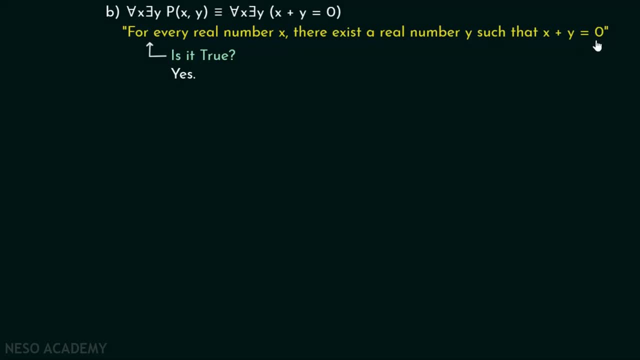 one real number, y, for which x plus y is equal to 0, right, You can choose any real number x. there is always a real number y for that x. Right, Such that x plus y is equal to 0.. Please note that y depends on x, right, We can choose. 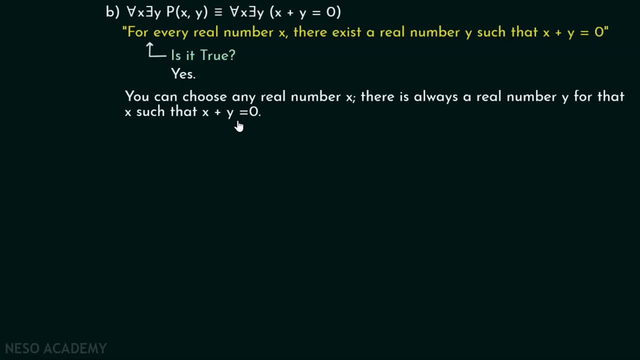 any real number x. It is our choice. There is always a real number y for that x, such that x plus y is equal to 0.. For example, you can consider x equal to 1.. You know that for x equal to 1,. 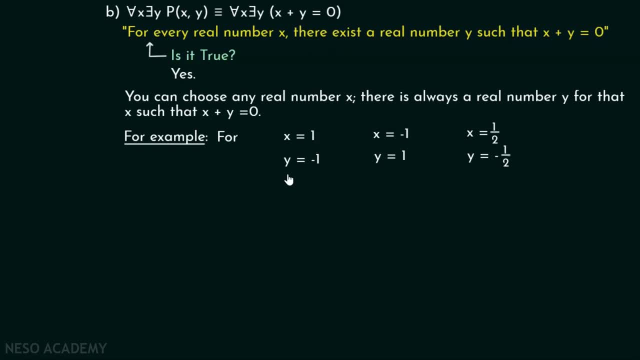 there is a y which makes x plus y 0,. right, We can choose y as minus 1.. Let's say, if we select x equal to minus 1, then we have y equal to 1.. If we choose x equal to 1 by 2,, then we have 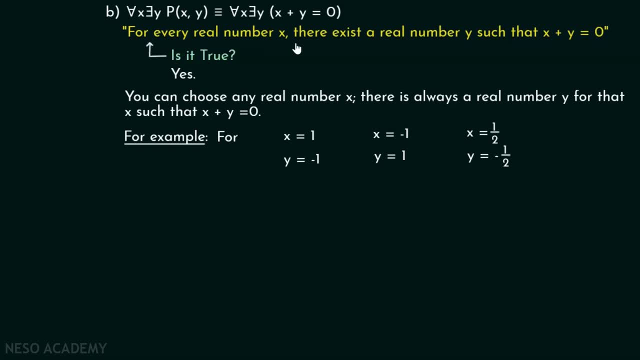 y equal to minus 1 by 2.. Now you get it Why: for every real number x there exists a real number y, such that x plus y equal to 0 is true. right, If you are confused, then you can follow these steps. 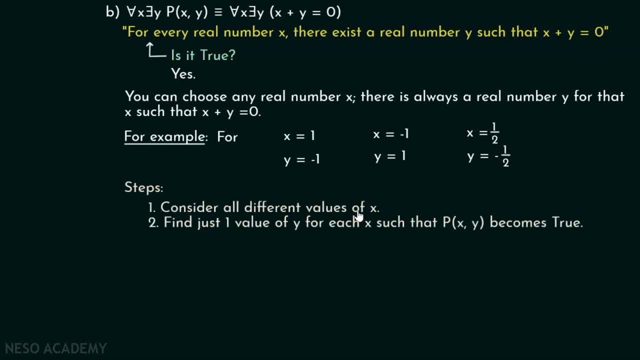 Consider all different values of x. okay, You should consider all different values of x, because it is for all x. right Now. you just have to find one value of y. okay, Because for all x, there exists y, There is a, there exists y written over here. You just have to find just one value. 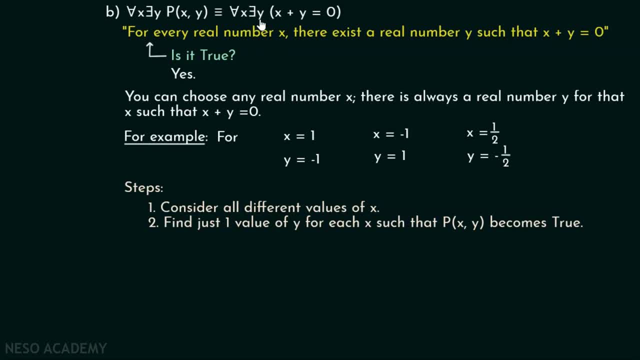 Okay, Because for all x, there exists y, There is a, there exists y written over here. You just have to find just one value of y for each x, such that pxy becomes true. These are the steps you can follow, Right. 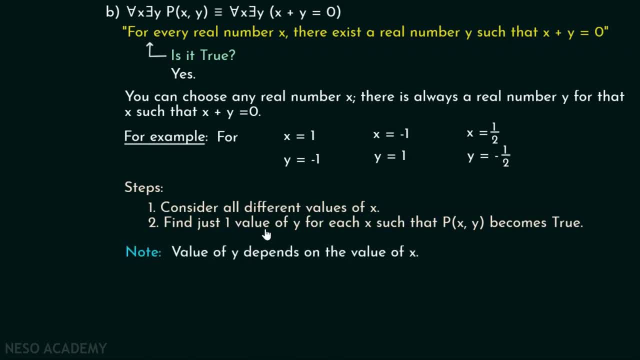 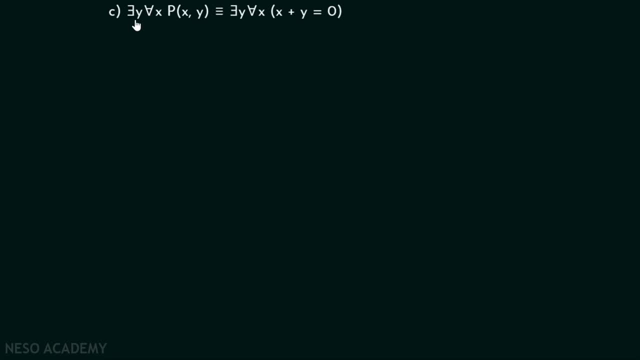 Please note that Value of y depends on the value of x. That is why I am saying we just have to find one value of y for each x. Okay, Now let's consider part c. There exists y for all x px. comma. y can be written as: 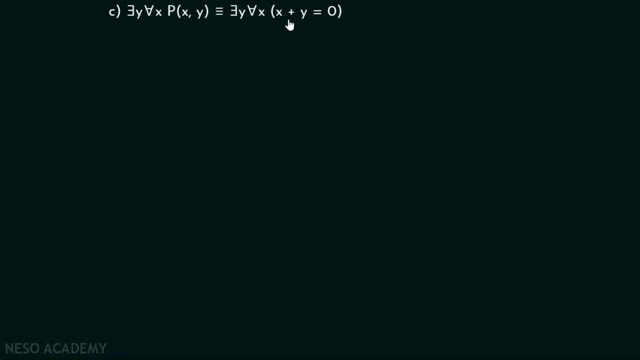 there exists y for all x, x plus y, equal to 0.. We can write this statement: as there exists some real number y, such that for every real number x, x plus y is equal to 0.. Isn't that so? There exists some real number y, such that for every real number x, x plus y is equal to 0.. 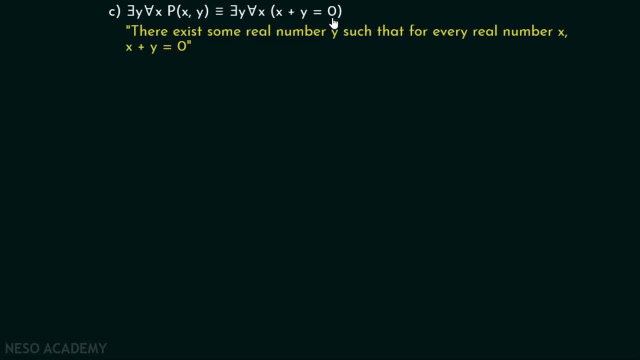 Isn't that? so There exists some real number, y, such that for every real number, x, x plus y, is equal to 0. Let me tell you this is different from what we have seen before, That is, for all x there exists y, x plus y is equal to 0. 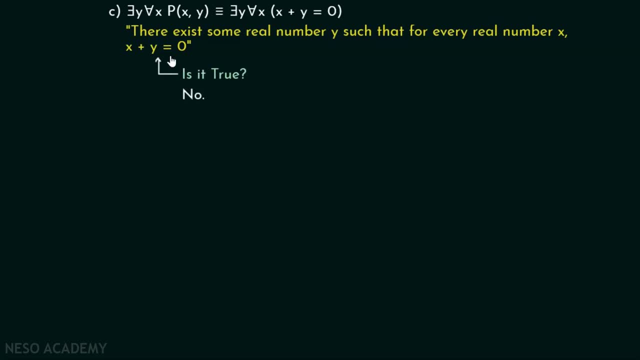 Okay, Now is it true? No, Let me tell you this is not true. It is asking us to find a real number y for which pxy becomes true by plugging in every real number x. Okay, So it is asking us to find some real number y. 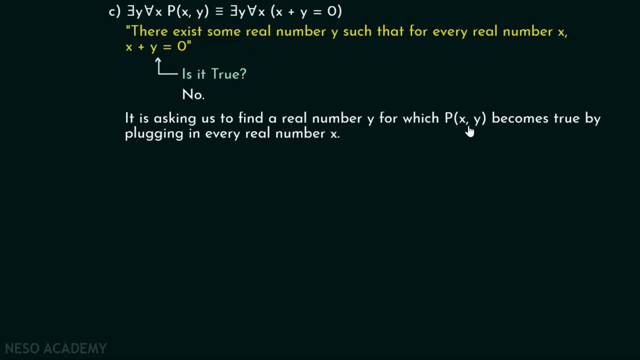 We just need one real number. Okay, For which pxy becomes true. For which pxy becomes true. Okay, For which pxy becomes true By plugging in every real number x. we have to plug in every real number x. 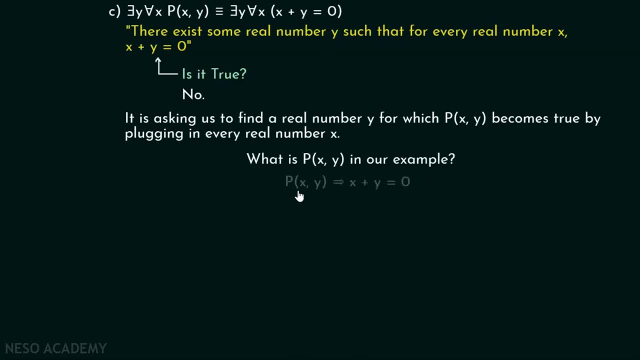 What is p? in our example It is x plus y equal to 0.. So we can write p as x plus y, equal to 0.. First take some real number, y. Let's take y is equal to 1.. Let's just plug this value of y in p. 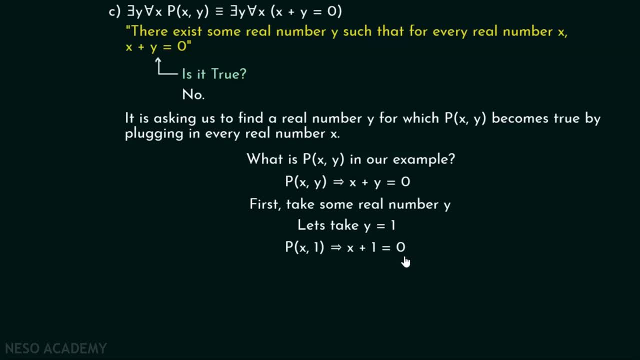 This becomes p, which can be written as x plus 1 equal to 0,. right, Now we have to plug in all real numbers x. Let's plug in 1 by 2.. We know that p is false, right? We also know p is also false. 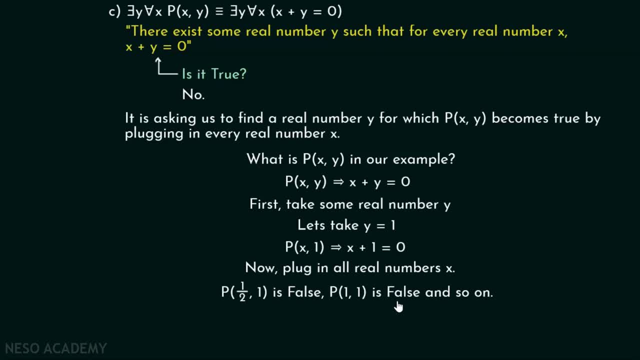 So it is clear from this fact that there is no real number y for which p becomes true. by plugging in every real number x, No matter what y you choose, p is always false for all real numbers x. Okay, I think this is clear to you. 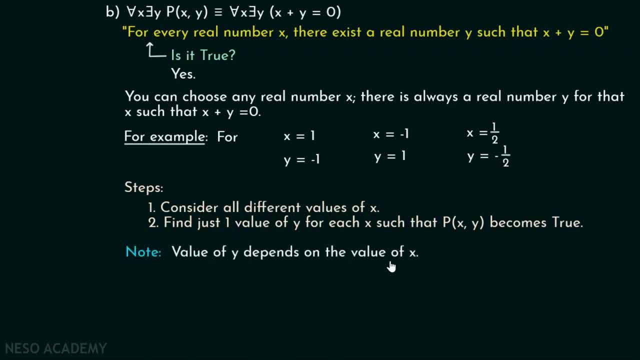 you can follow right. Please note that value of y depends on the value of x. That is why I am saying we just have to find one value of y for each x. okay, Now let's consider part c. There exists y for all x. px. comma y can be written as: there exists y for all x, x plus y equal to 0.. 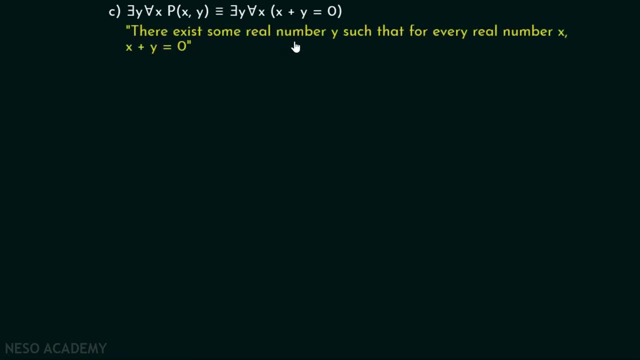 We can write this statement, as there exists some real number, y, such that for every real number, x, x plus y is equal to 0.. Isn't that so Number y, such that for every real number x, x plus y is equal to 0.. Let me tell you this is: 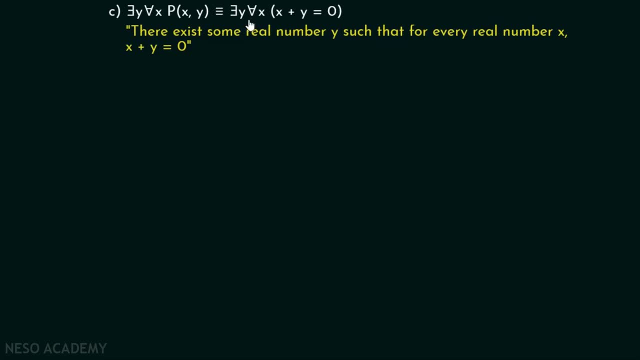 different from what we have seen before. That is, for all x, there exists y, x plus y, equal to 0,. okay, Now is it true? No, let me tell you, this is not true. It is asking us to find a real number. 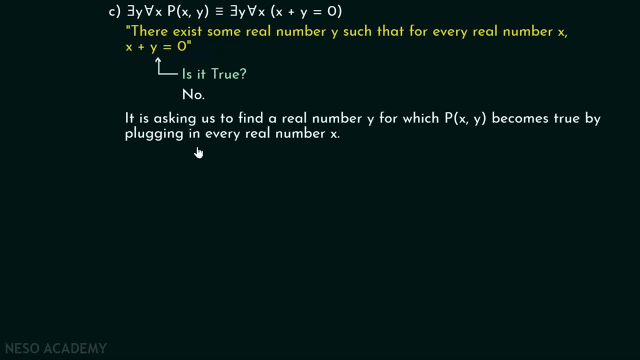 y, for which pxy becomes true by plugging in every real number x. okay, So it is asking us to find some real number y. We just need one real number, okay, For which pxy becomes true by plugging in every real number x. We have to plug in every real. 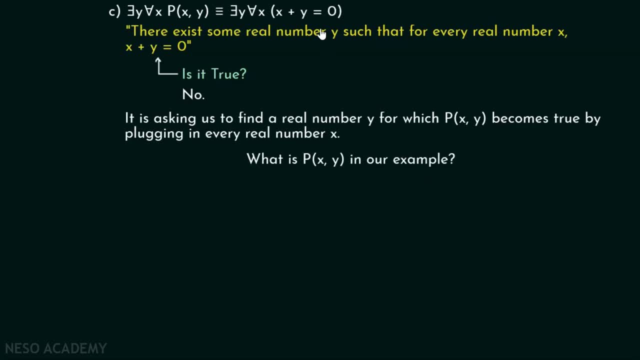 number x. What is pxy? in our example It is x plus y equal to 0. So we can write pxy as x plus y equal to 0.. First take some real number, y. Let's take y is equal to 1.. Let's just plug this value. 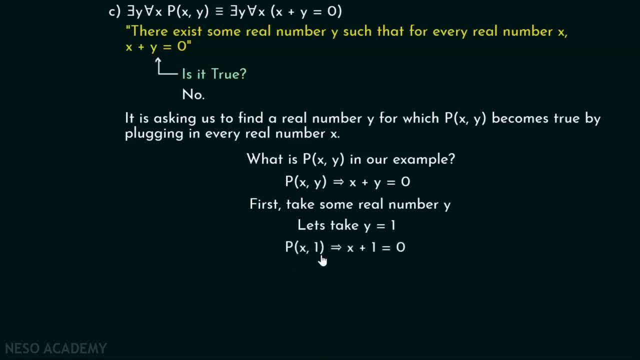 of y in px comma y. This becomes px comma 1, which can be written as x plus 1 equal to 0, right Now all real numbers x. Let's plug in 1 by 2.. We know that p1 by 2 comma 1 is false, right? We also know. 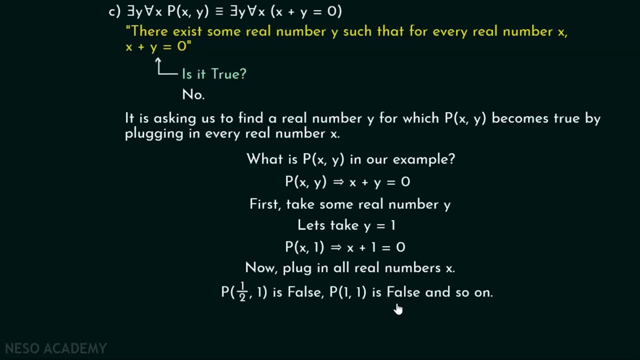 p1, comma 1 is also false. So it is clear from this fact that there is no real number y for which pxy becomes true. by plugging in every real number x, No matter what y you choose, px, comma y is always false for all real numbers x. okay, I think this is clear to you. Now let's just consider: 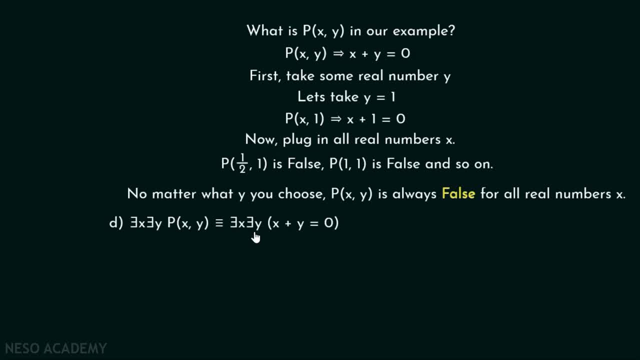 px comma y, px comma y can be written: as there exists x, there exists y, x plus y equal to 0, right, You can write this statement as there exists some real numbers, x and y, such that x plus y is equal to 0.. Isn't that so? Is it true? Obviously it is true, right, There exists some combination.